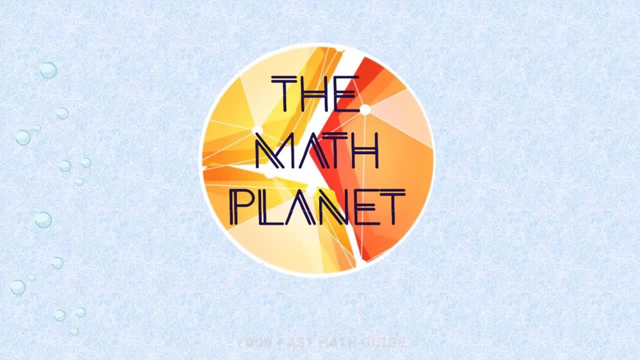 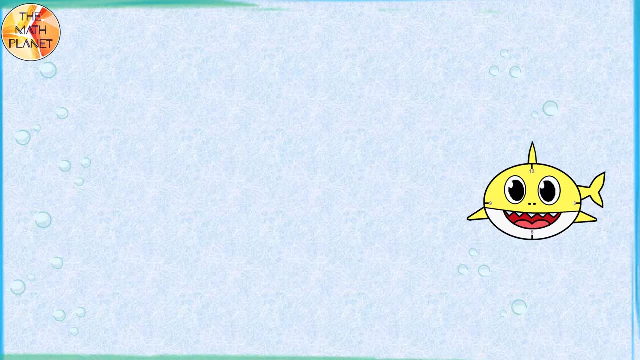 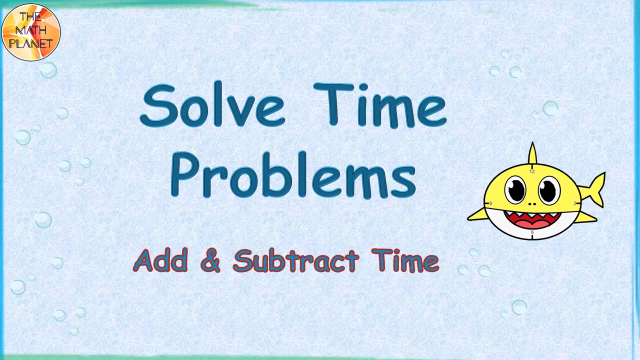 Welcome to the Math Planet, your fast math guide. Hi everyone, Baby Shark is on time today. He will teach you how to solve time problems. In this video, you will learn how to add and subtract time. So let's get started. 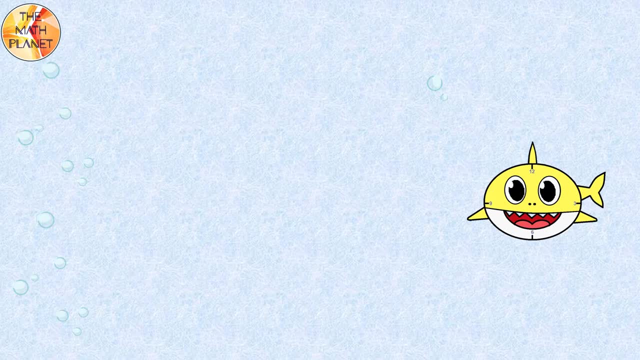 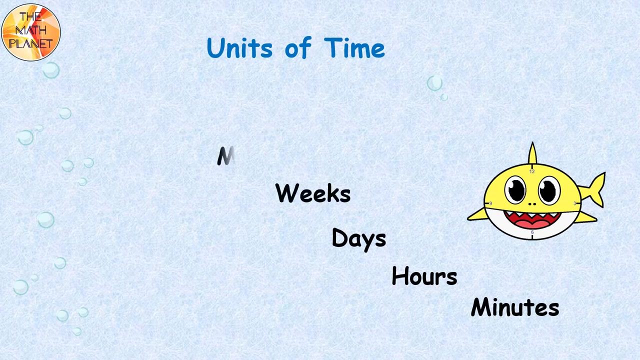 Hello, my dear friends, Today I'll show you how to solve time word problems that involve addition and subtraction. We will include the following units of time: Minutes, Hours, Days, Weeks, Months and Years. The rules that we will study are: 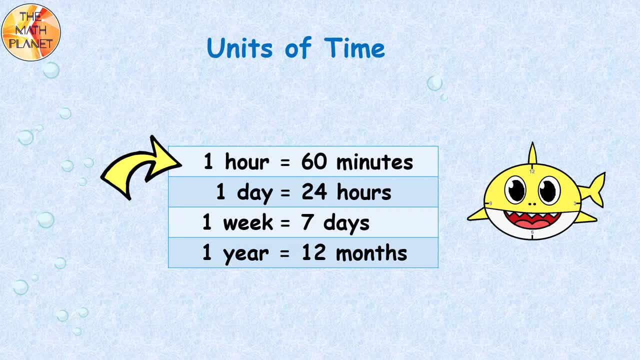 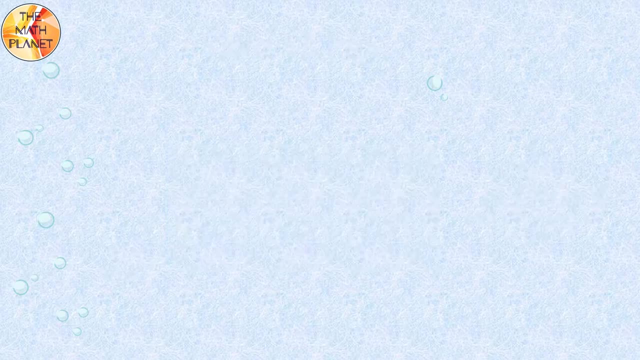 1 hour equals 60 minutes, 1 day equals 24 hours, 1 week equals 7 days and 1 year equals 12.. Our first word problem involves hours and minutes. Let's read question 1.. Henry's flight lasts 1 hour 40 minutes. 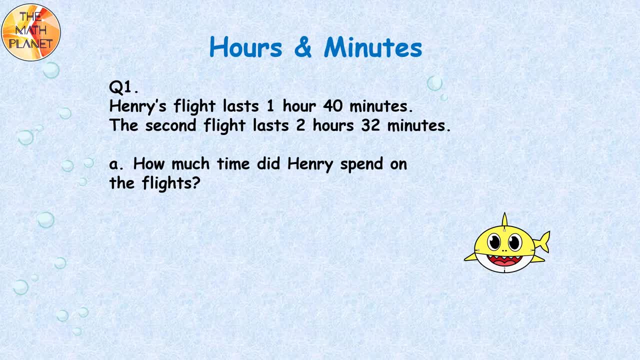 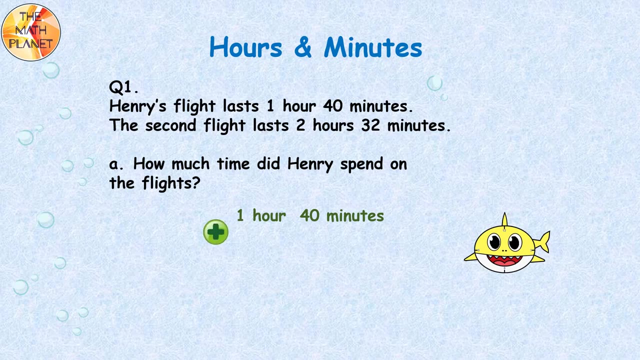 The second flight lasts 2 hours 32 minutes. How much time did Henry spend on the flight? We will add the times for both flights, So our equation will be 3 hours 72 minutes plus 2 hours 32 minutes. 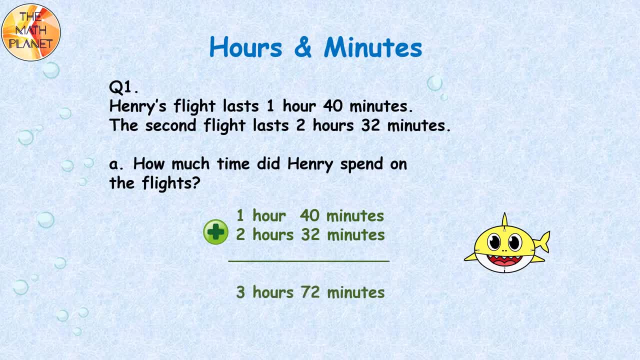 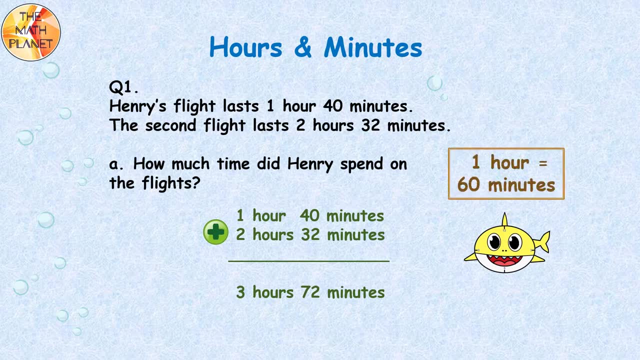 The sum will be 3 hours 72 minutes, But we already know that 1 hour equals 60 minutes. Since 72 minutes is greater than 1 hour, we will regroup 60 minutes as 1 hour. So the sum will be 4 hours and 12 minutes. 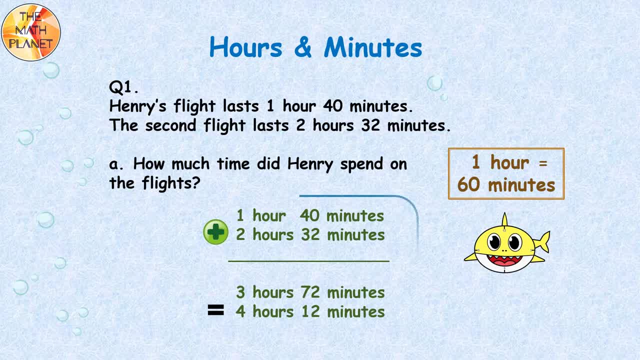 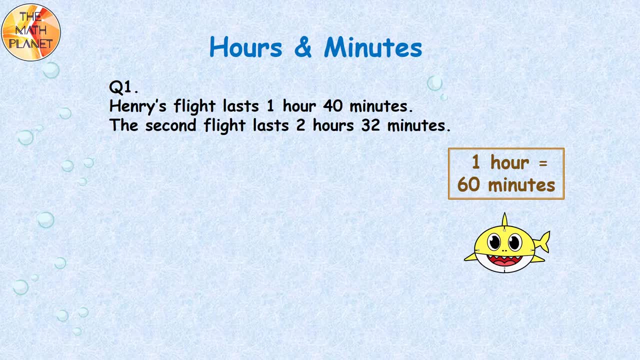 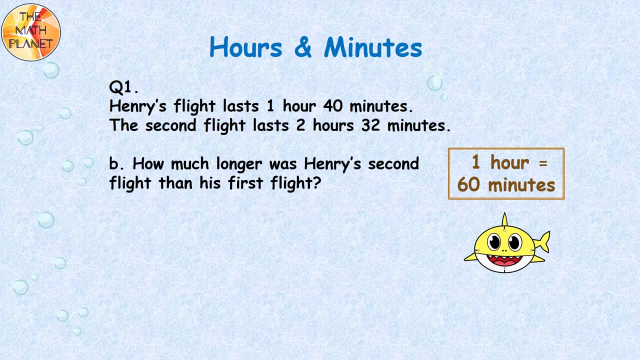 And we can say that Henry spent 4 hours 12 minutes on both flights. Now we need to answer question B: How much longer was Henry's second flight than his first flight? We will subtract the last time from the greater time. 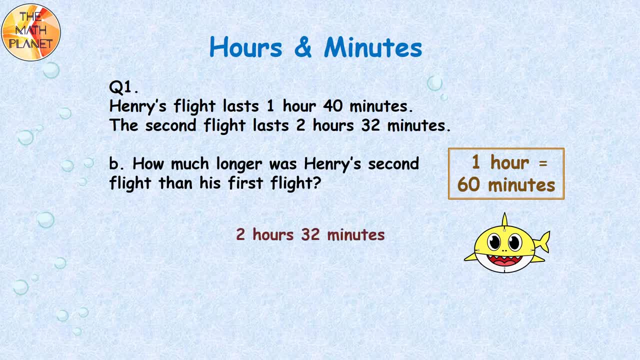 So our equation will be 2 hours 32 minutes minus 1 hour 40 minutes And we will start subtracting from the greater time, We will start subtracting from the minutes part. What is 32 take away 40?. 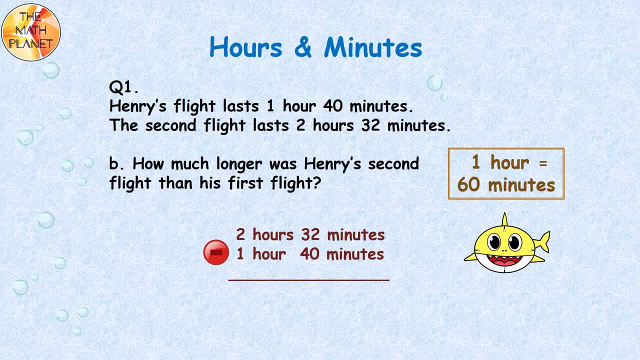 We cannot subtract 40 from 32.. So we need to regroup. So we will cross 32 minutes and we will also cross the 2 hours And we will regroup according to the rule: 1 hour equals 60 minutes. 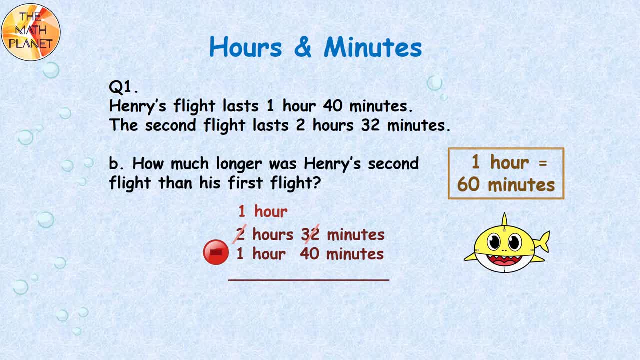 When we take away 1 hour, we will have 1 hour left And we will add 60 minutes to the 32 minutes, So we will have 32 minutes. So we will have 32 plus 60 equals 92 minutes. 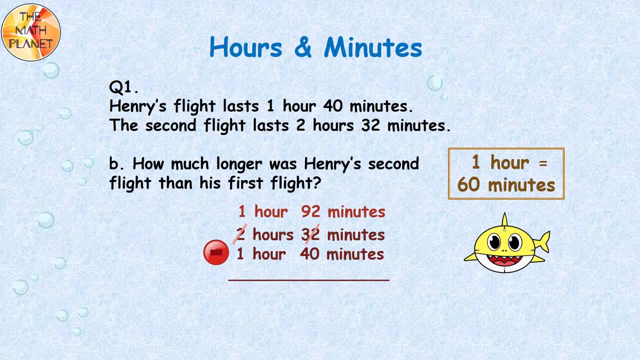 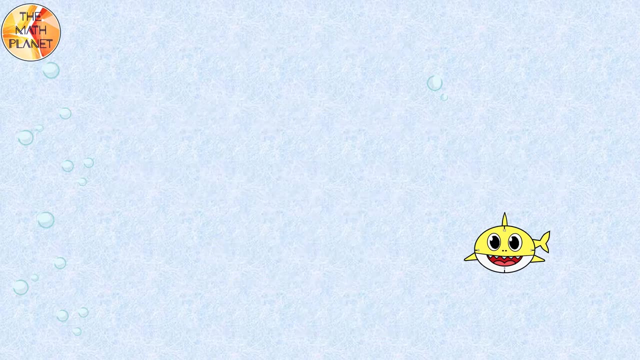 Then we can subtract 1 hour 92 minutes minus 1 hour 40 minutes equals 52 minutes. This means that Henry's second flight was 52 minutes longer than his first flight. Our second word problem involves days and hours. Let's read question 2.. 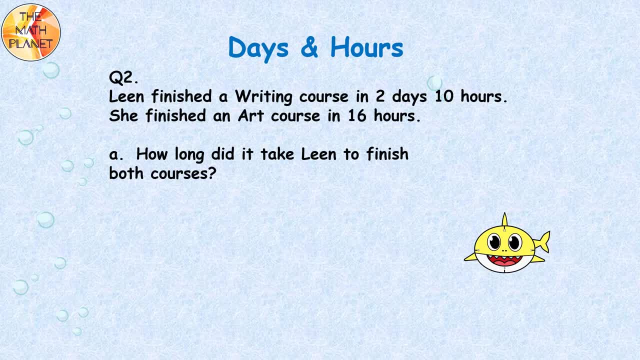 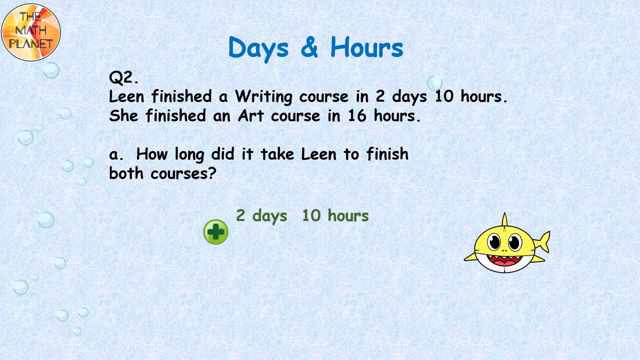 Henry finished a writing course in 2 days 10 hours. She finished an art course in 16 hours. How long did it take Lynn to finish both courses? We will add the times for both courses, So our equation will be 2 days, 10 hours plus 16 hours. 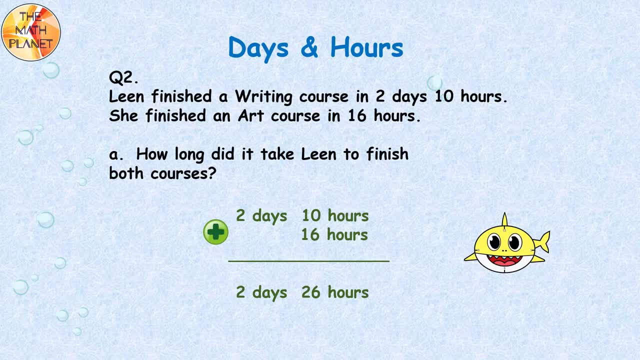 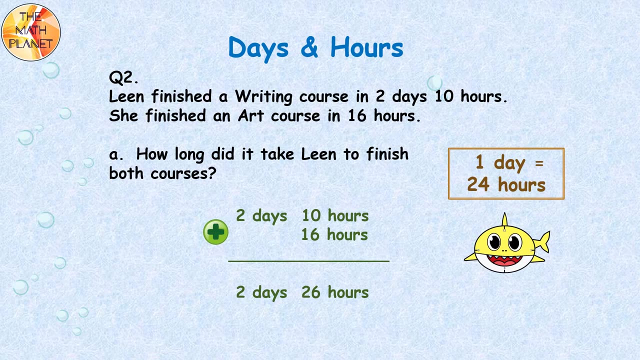 And the sum will be 2 days, 26 hours, But we know that 1 day equals 24 hours. Since 26 hours is greater than 1 day, we will regroup, We will take away 24 hours and we will add 1 day instead. 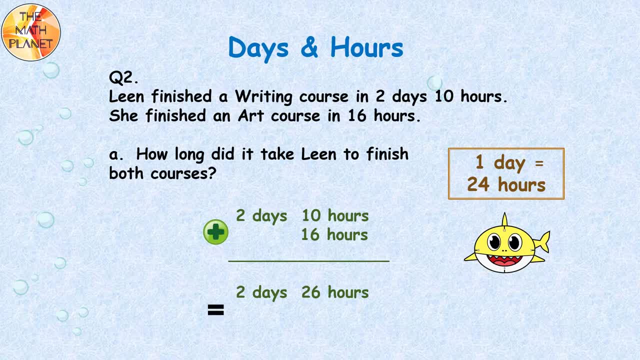 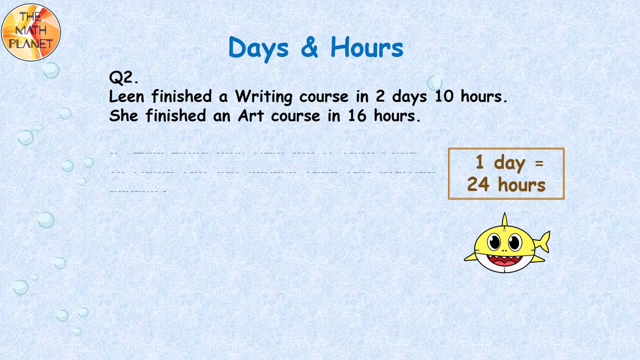 So the sum will be 3 days and 2 hours, And we can say that Lynn took 3 days and 2 hours to finish both courses. Now let's solve question b: How much less time did it take Lynn to finish the art course than the writing course? 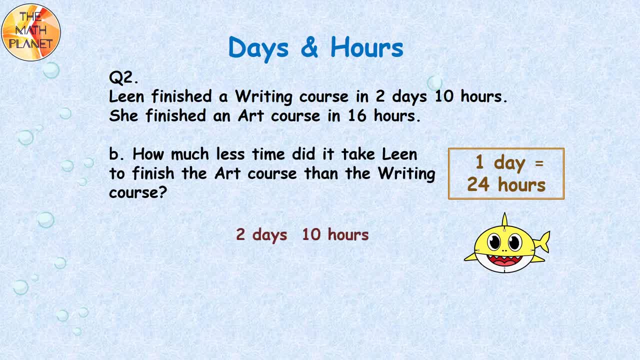 Let's write the subtraction equation: 2 days, 10 hours minus 16 hours. We will start subtracting from the hours. What is 10 minus 16?? We cannot take away 16 from 10.. So we will regroup. 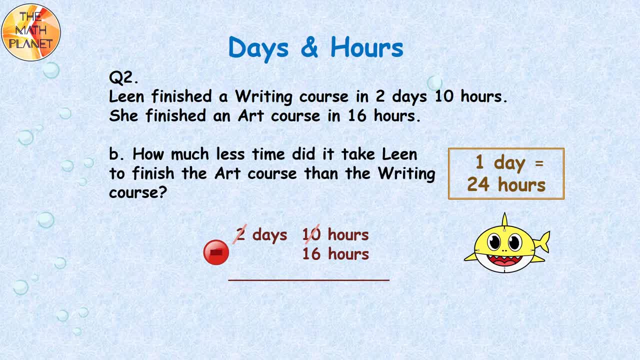 We will cross 10 hours and we will cross the 2 days and we will regroup according to the rule 1 day equals 24 hours. When we take away 1 day, we will have 1 day left And we will add 24 hours. 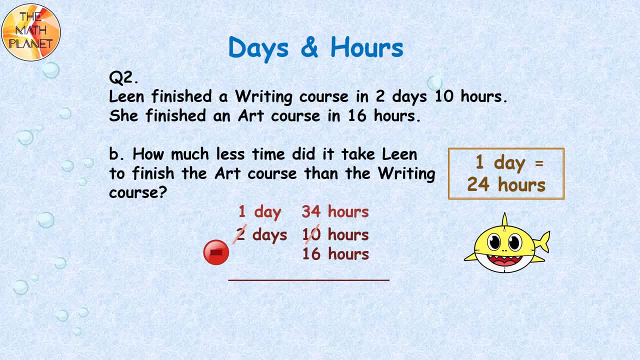 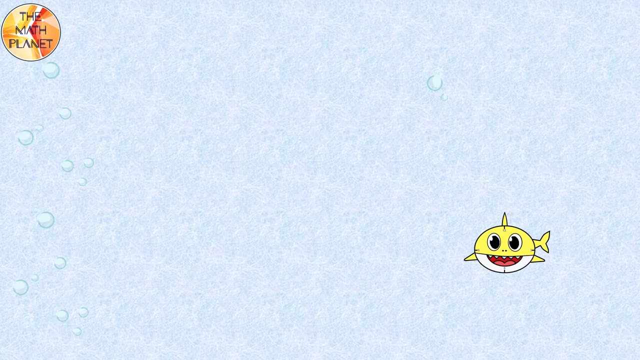 So we will have 34 hours Now the difference will be 1 day and 18 hours. Our third word problem involves weeks and days. Let's read question 3.. Grandma knitted a scarf in 1 week, 5 days. 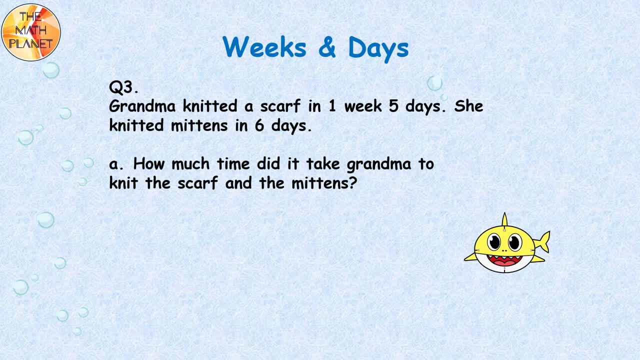 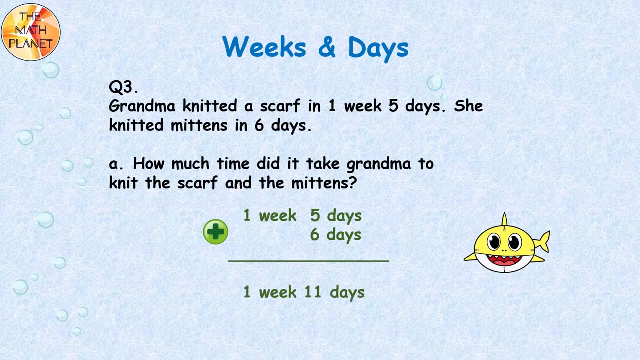 She knitted mittens in 6 days. How much time did it take grandma to knit the scarf and the mittens? Let's write the addition equation: 1 week 5 days plus 6 days, The sum will be 1 week, 11 days. 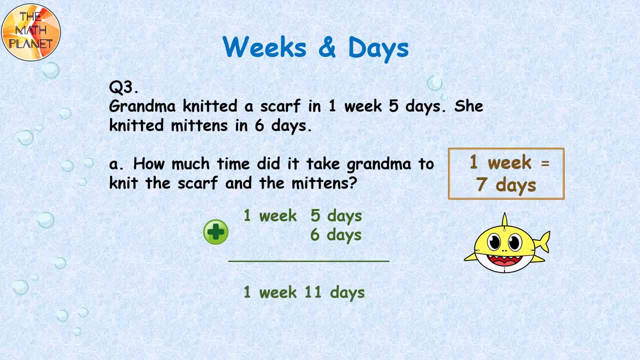 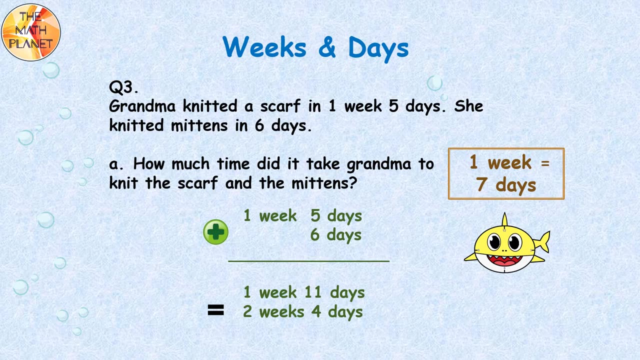 But we know that 1 week equals 7 days. Since 11 days is greater than 1, we regroup 7 days into 1 week. So the sum will be 2 weeks, 4 days. So grandma knitted the scarf and the mittens in 2 weeks, 4 days. 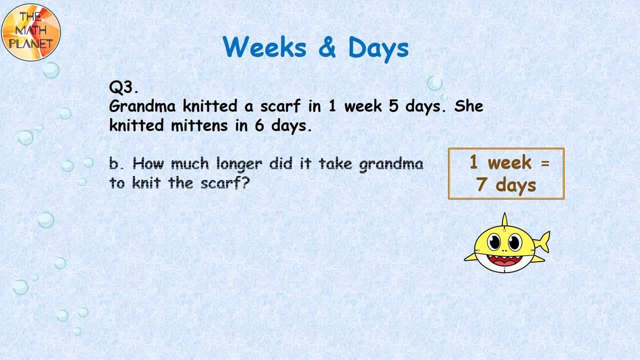 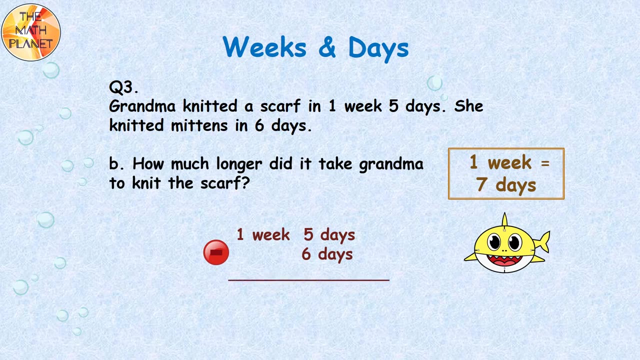 Now let's answer question b: How much longer did it take grandma to knit the scarf? The subtraction equation is 1 week, 5 days minus 6 days, 6 days, And we start subtracting from the days. What is 5 minus 6?? 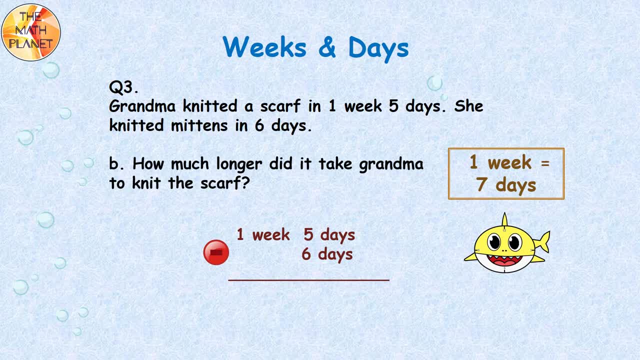 We cannot take away 6 from 5.. So we will regroup, We cross the 5 days and we cross the 1 week, And we follow the rule: 1 week equals 7 days, So we will have 0 weeks left. 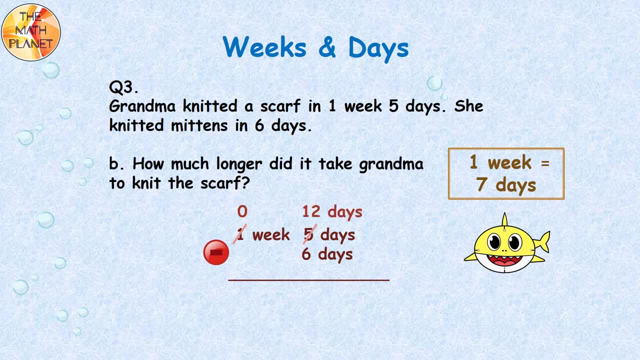 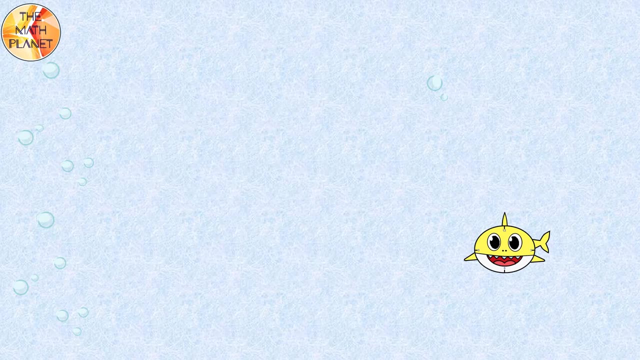 And the days will be 5 plus 7 equals 12 days, And the difference is 12 minus 6 equals 6 days. So we conclude that the scarf took 6 more days than the mittens. Our last word problem involves years and months. 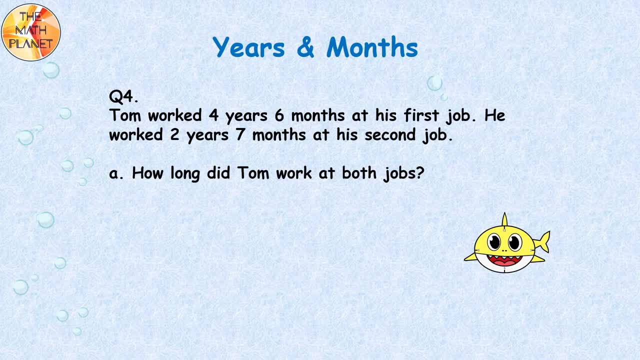 Let's read question 4.. Tom worked 4 years 6 months at his first job. He worked 2 years 7 months at his second job. How long did Tom work at both jobs? Let's write the addition equation: 4 years 6 months. 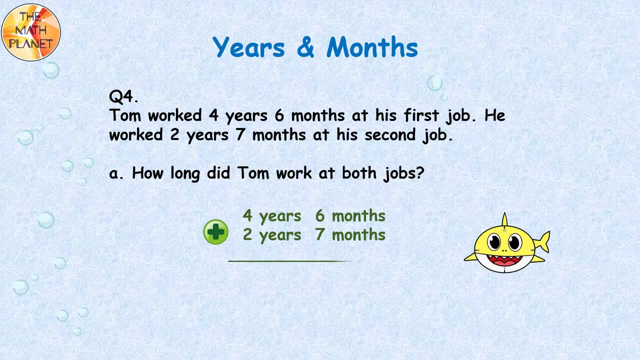 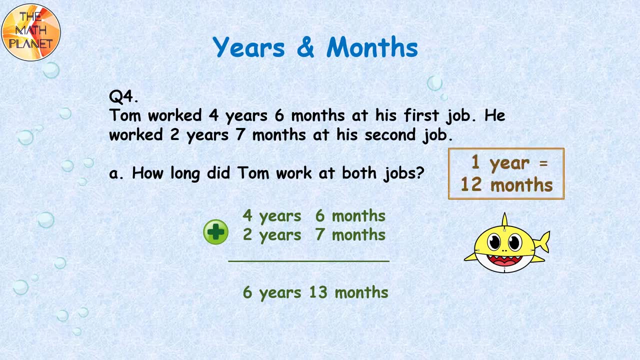 plus 2 years, 7 months And the sum will be 6 years 13 months. But we know that 1 year equals 12 months. Since 13 months is greater than 1 year, we regroup 12 months into 1 year. 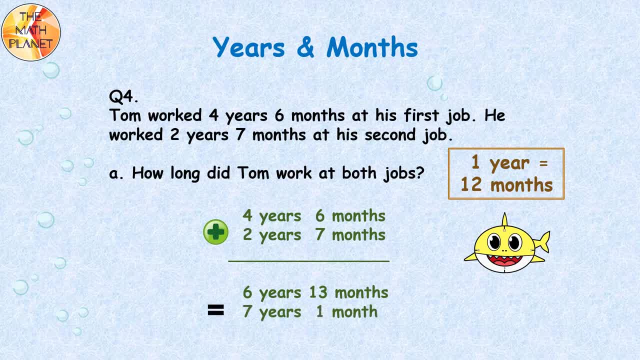 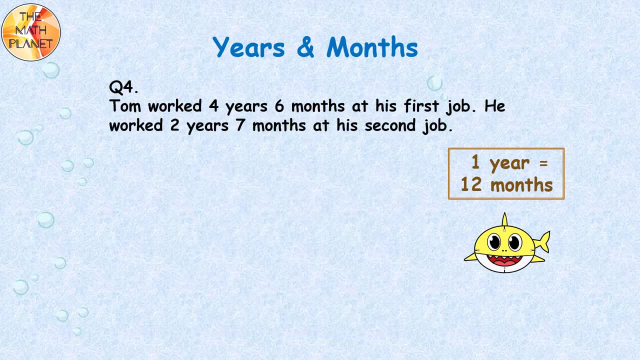 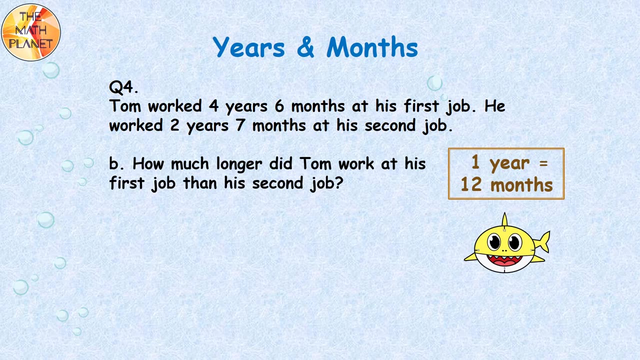 And the sum will be 7 years and 1 month. So Tom worked a total of 7 years and 1 month at both jobs. Now let's answer question B: How much longer did Tom work at his first job than his second job? 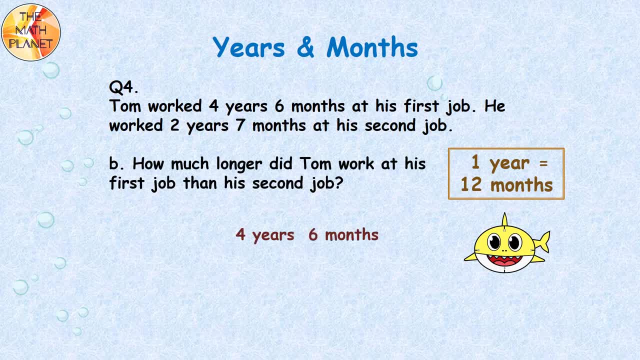 Let's write the subtraction equation: 4 years, 6 months minus 2 years, 7 months, And we'll start subtracting from the months. What is 6 minus 7?? We cannot take away 7 months from 6 months, So we regroup. 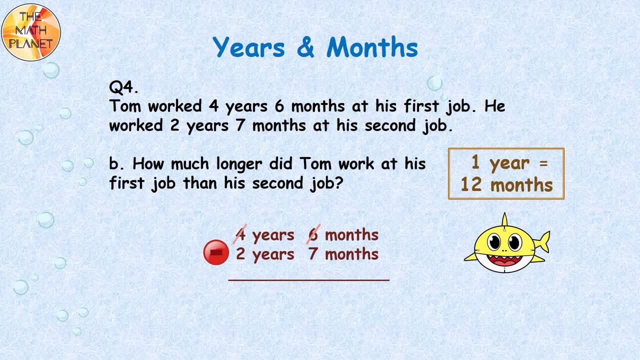 We cross the 6 months and we cross the 4 years. We regroup according to the rule: 1 year equals 12 months, So when we take away 1 year, we will have 3 years left And the months will be. 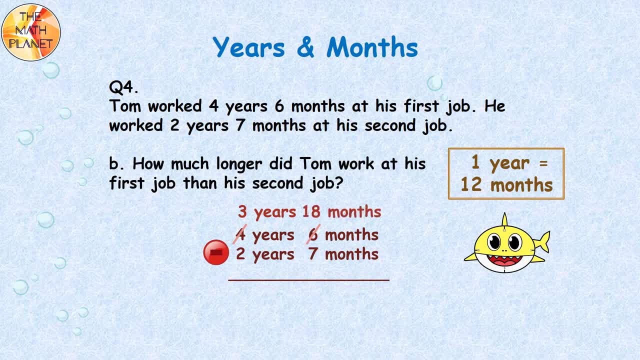 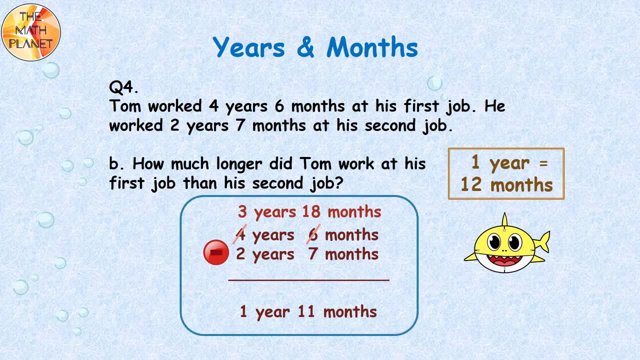 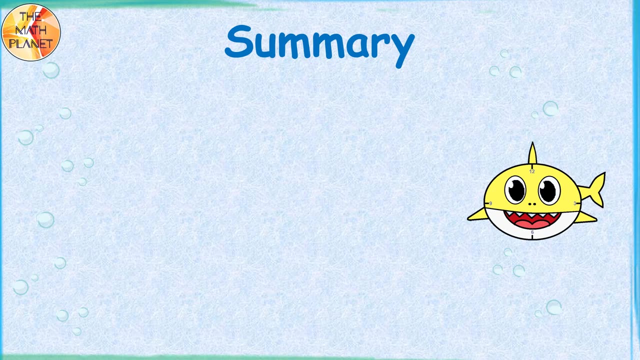 6 plus 12 equals 18 months, And the difference is 1 year 11 months. So Tom worked 1 year 11 months longer at his first job. To sum up, today we solved word problems that involve adding and subtracting time. 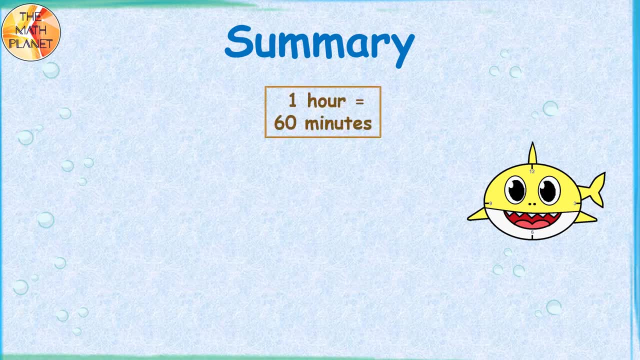 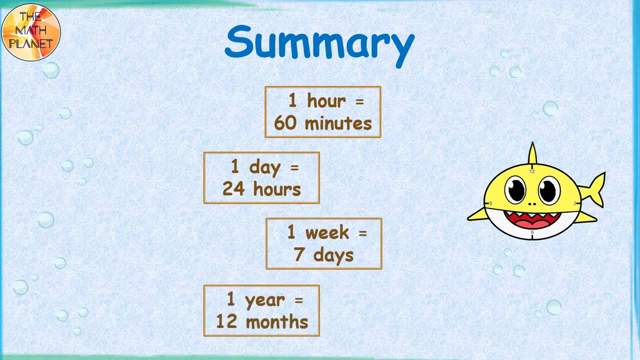 The rules that we used in this video are: 1 hour equals 60 minutes, 1 day equals 24 hours, 1 week equals 7 days And 1 year equals 12 months. That's all for today. Thanks for watching The Math Planet. 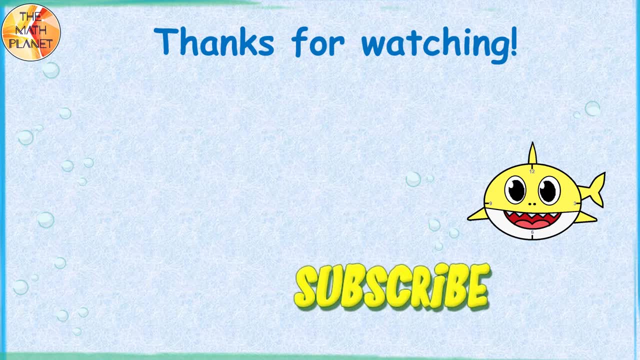 Don't forget to subscribe for more videos. See you next time.